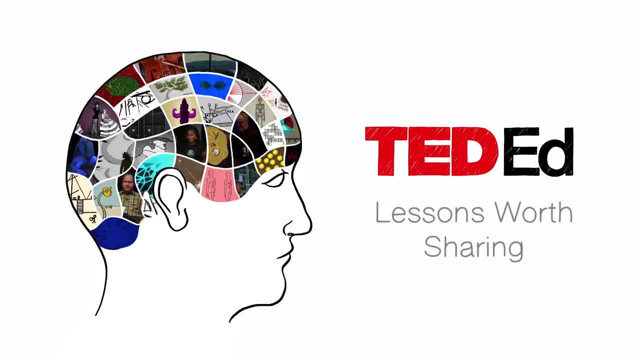 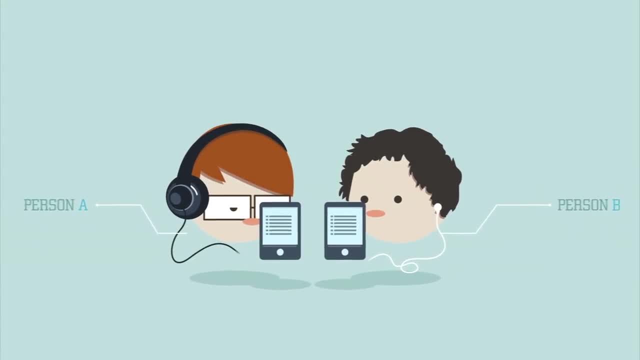 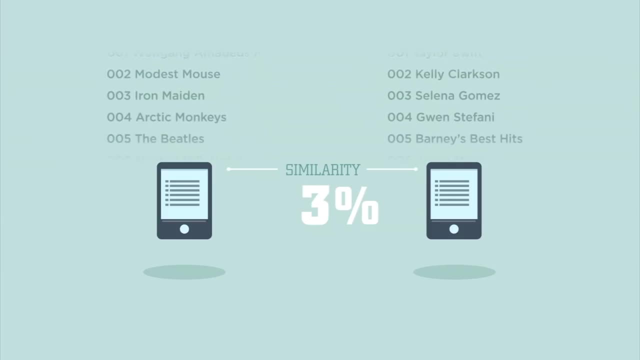 Imagine two people are listening to music. What are the odds that they are listening to the exact same playlist? Probably pretty low. After all, everyone has very different tastes in music. Now what are the odds that your body will need the exact same medical care and treatment? 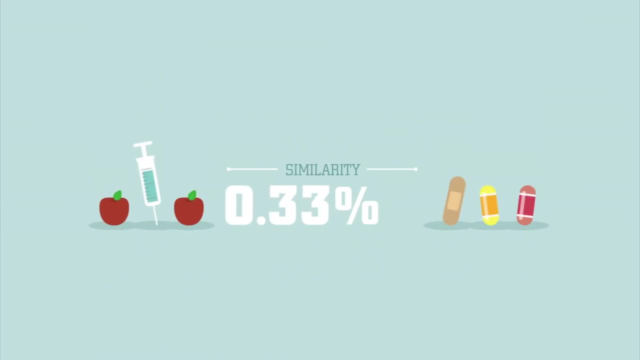 as another person's body Even lower As we go through our lives. each of us will have very different needs for our own health care. Scientists and doctors are constantly researching ways to make medicine more personalized. One way they are doing this is by researching stem cells. 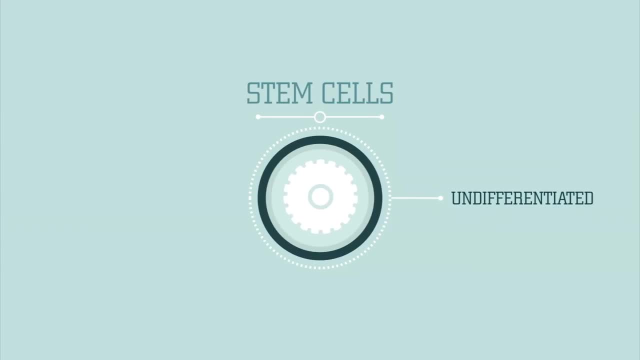 Stem cells are cells that are undifferentiated, meaning they do not have a specific job or function. While skin cells protect your body, muscle cells contract and nerve cells send signals, stem cells do not have any specific structures or functions. Stem cells do have the potential to become all other kinds of cells in your body. Your body uses. 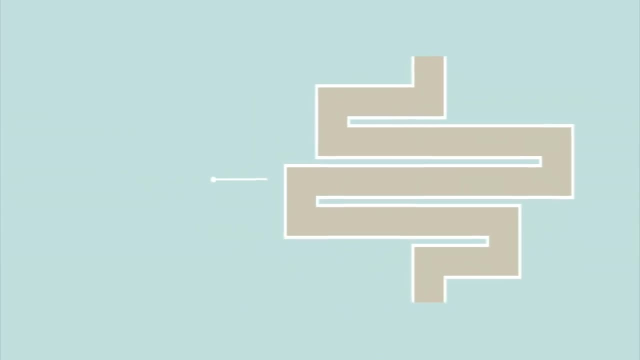 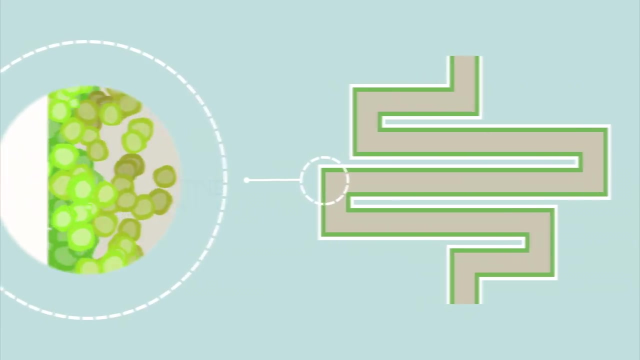 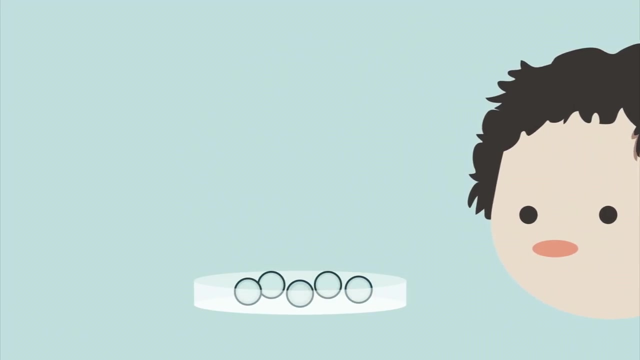 stem cells to replace worn-out cells when they die. For example, you completely replace the lining of your intestines every four days. Stem cells beneath the lining of your intestines replace these cells as they wear out. Scientists hope that stem cells could be used to create a 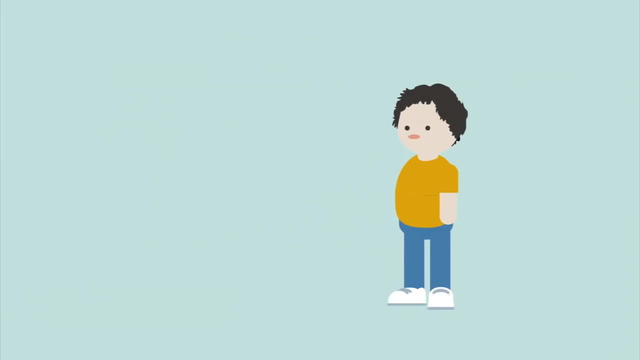 very special kind of personalized medicine in which we could replace your own body with a body part, with, well, your own body parts. Stem cell researchers are working hard to find ways in which to use stem cells to create new tissue to replace the parts of organs that are damaged. 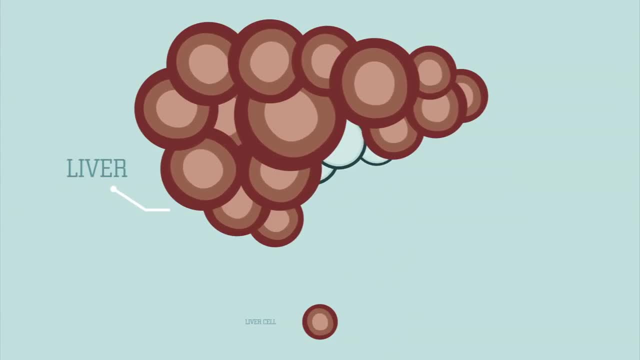 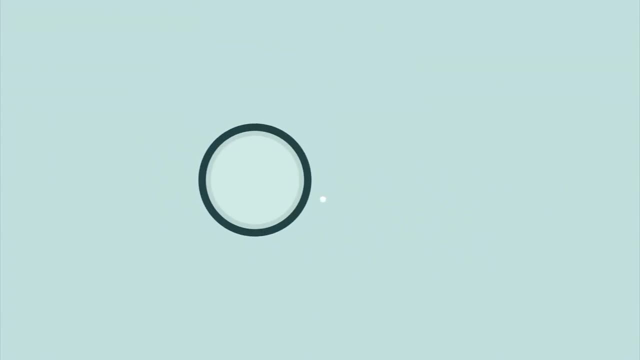 by injury or disease. Using stem cells to replace damaged bodily tissue is called regenerative medicine. For example, scientists currently use stem cells to treat patients with blood diseases such as leukemia. Leukemia is a form of cancer that affects the body. Stem cells are used to. 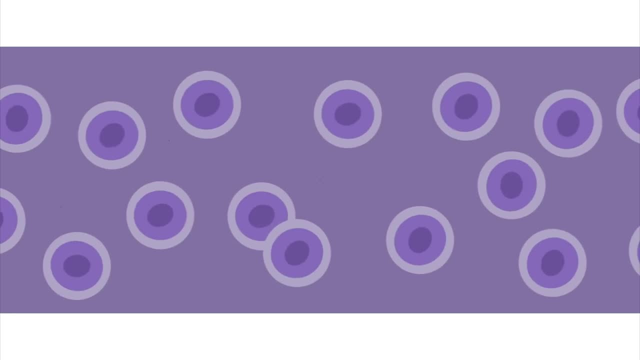 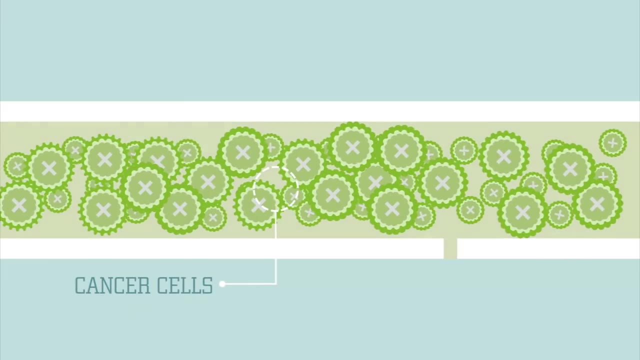 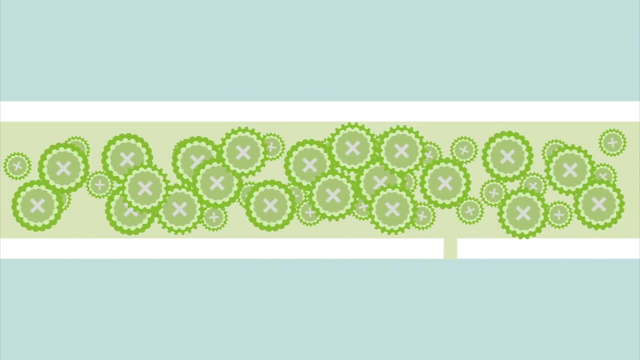 create new tissue that affects your bone marrow. Bone marrow is the spongy tissue inside your bones where your blood cells are created. In leukemia, some of the cells inside your bone marrow grow uncontrollably, crowding out the healthy stem cells that form your blood cells. Some leukemia